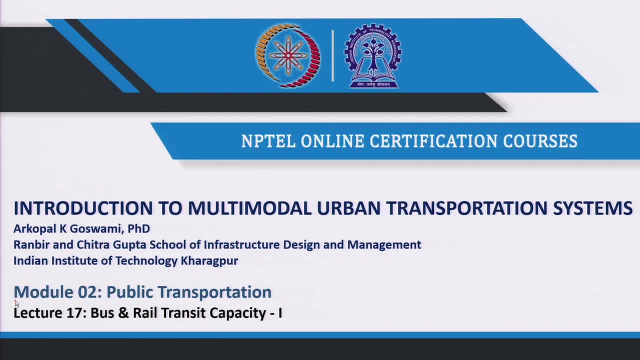 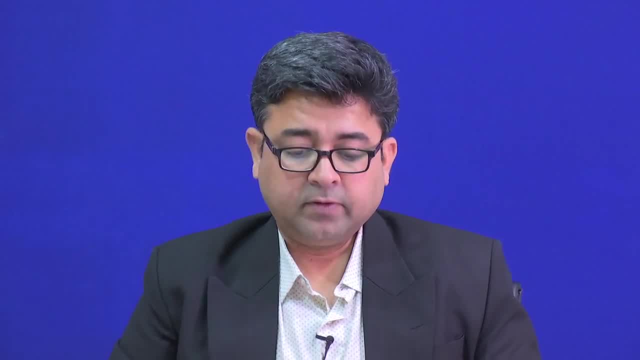 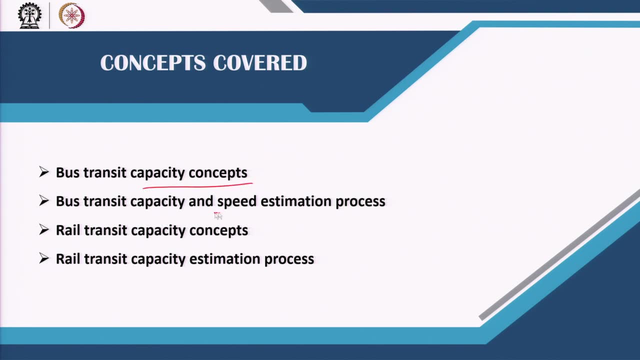 the. I have two parts of this lecture. In the second part of the lecture I will be looking into different types of solved examples. In this part we will introduce you to the concepts of bus transit capacity And we will look at how capacity and speed estimation 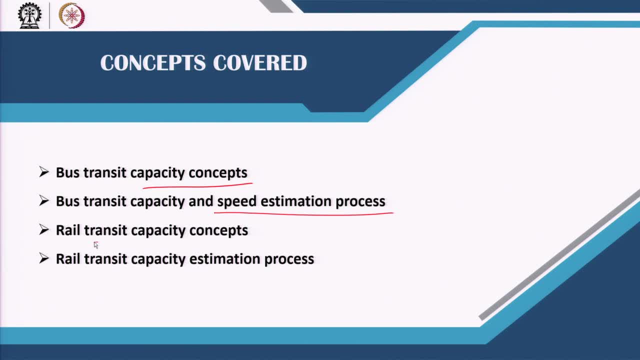 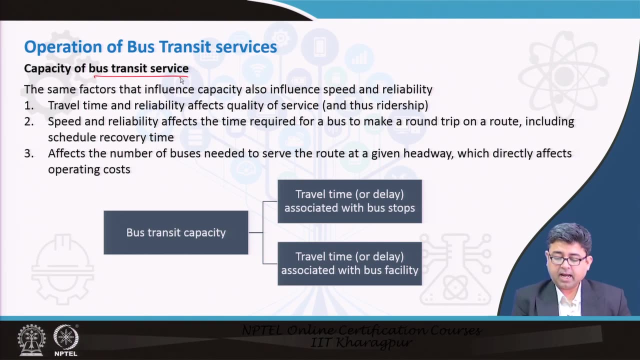 process is carried out. Similarly, we will be looking at transit, at rail transit capacity concepts and look at how rail transit capacity estimation process is carried out. So, when we are talking about the capacity of a bus transit service system, we are looking at travel time, capacity based on travel time and capacity based on travel time or delay. 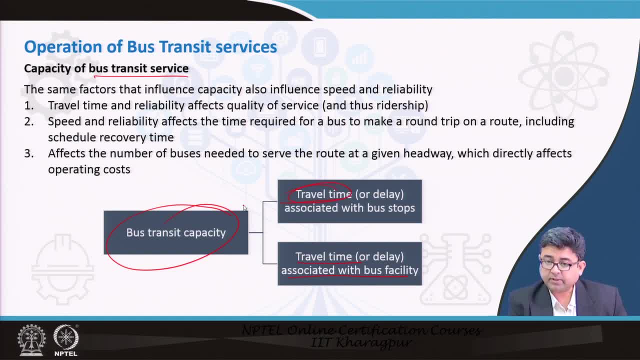 associated with bus facility. So travel time is something that we are looking at: Travel time with bus stops or travel times with bus facilities- See travel time. so this is something that you have to. you have to start understanding that the capacity of a 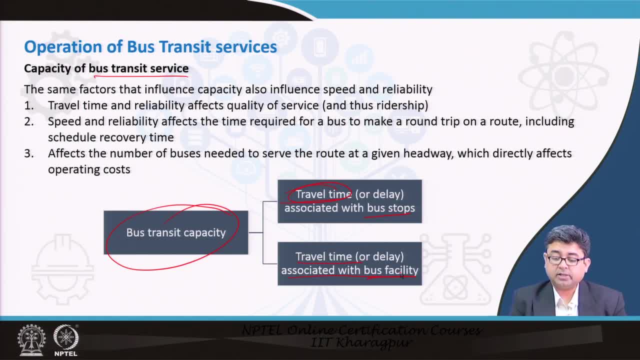 public transportation system can be measured using time. So capacity usually we think is the number of people that you can fit in in your bus service, but usually it is the number of people that crosses a certain point in your bus service. So usually it is the 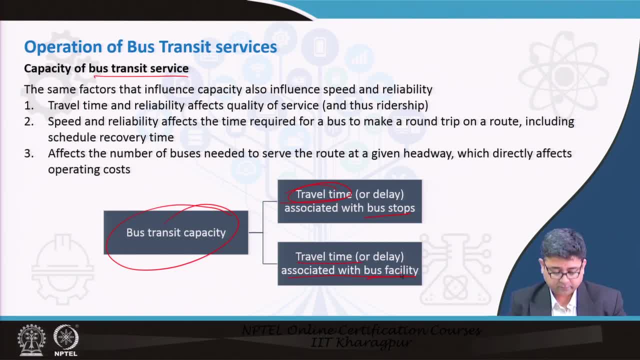 point in a given amount of time. right. Remember the definition of speed and travel time right. Travel time and reliability affects the quality of service. If you are not, if you have unreliable travel times or if you have very high travel times, then people will not ride your public. 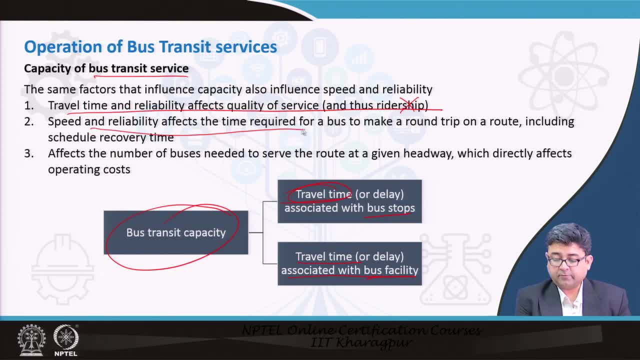 transportation system. Speed and reliability affects the time required for a bus to make a round trip as well. So from a user's point of view and an operator's point of view, you see they all impact the public transportation system It they also affects the number of buses needed to be served on that road, on that. 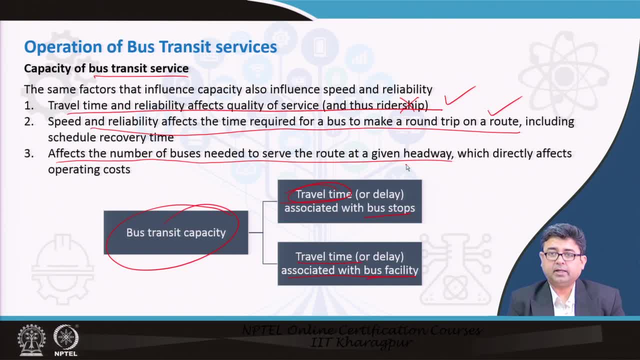 route, given a specific headway that it has to maintain right. If the, if the, if the travel time taken is too much between two stops, then there has to be more number of buses that have to be in operation, and that increases the operation cost as well. 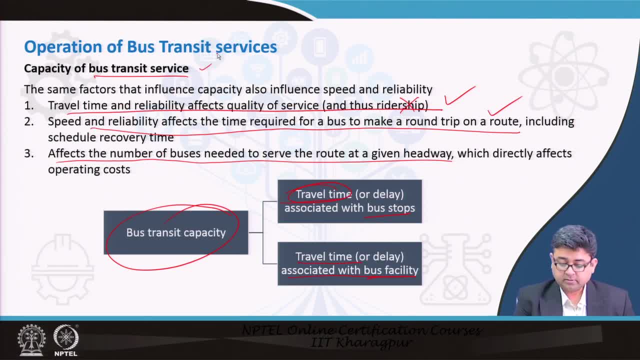 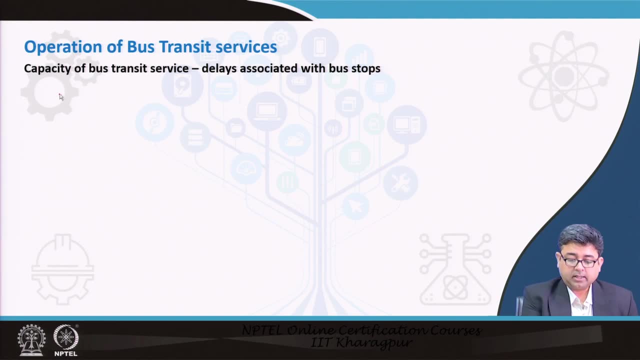 So capacity of ah bus transit service can be looked at from the point of view of travel time and travel time at ah, which locations the travel time at bus stops or travel time with a bus facility. So let us look at ah capacity of a bus transit. 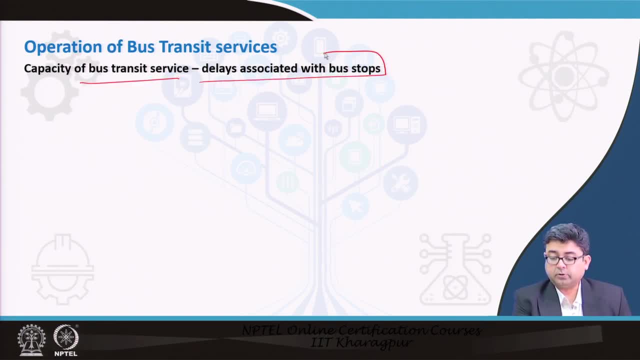 service and look at what are delays associated with the bus stops. So look at, look it from the point of view of bus stops and how you can minimize those delays to ah maximize the capacity. So usually at the bus stops, ah buses decelerate the time spent slowing down to serve the stop. 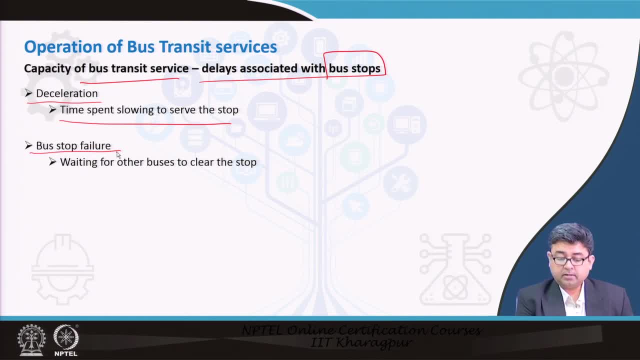 ah, there may be ah bus stop failure, So waiting for other buses to clear the stop right Maybe ah there is no space ah for this incoming bus to stop because there are other buses that are already ah at the bus stop ah boarding last time. waiting for passengers. 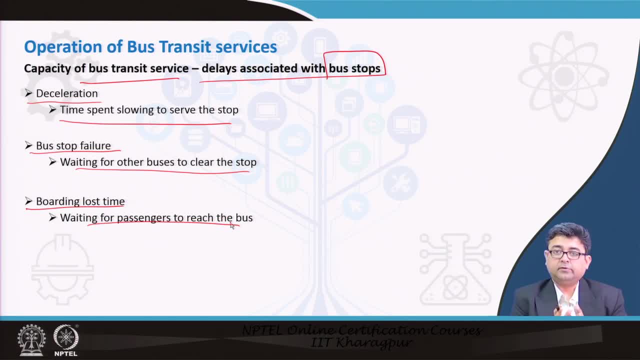 to reach the bus. ah, If, ah, you are not. ah, if you, if you do not have a bus bay, then you are. then you are waiting, ah, on the pavement and there is some time, ah, time lag, that happens- for the passengers to come out of the bus stop. come on to the pavement and then access. 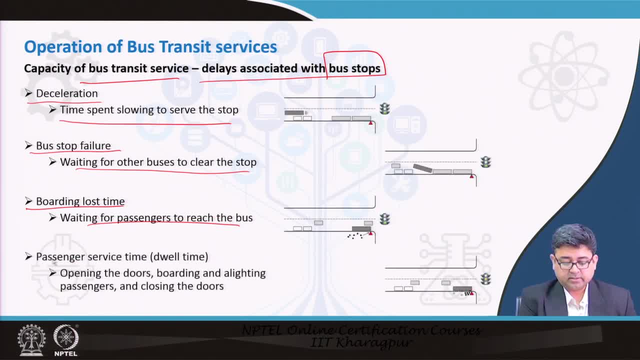 the bus that is boarding last time, and then passenger service time, which is the dwell time, which you already know about, right? So deceleration is the bus is coming, ah, and so, ah, it has to, ah, lower its speed. ah, ah, bus stop failure, ah, it cannot get in there because 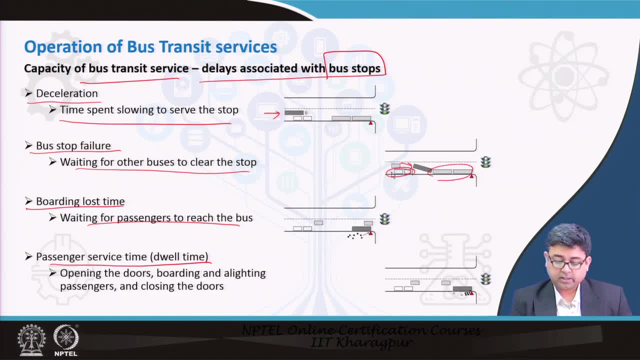 there are parked vehicles and 2 buses are already being served, So it cannot get in there. boarding last time ah. Now there are the lots of people already ah boarding another bus ah, or they cannot reach ah this bus in time. and then ah the actual dwell time which are needed by the 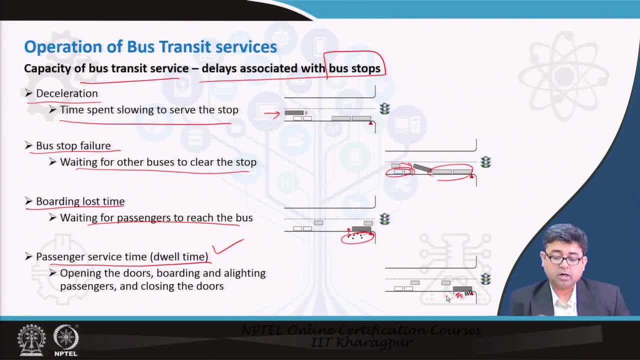 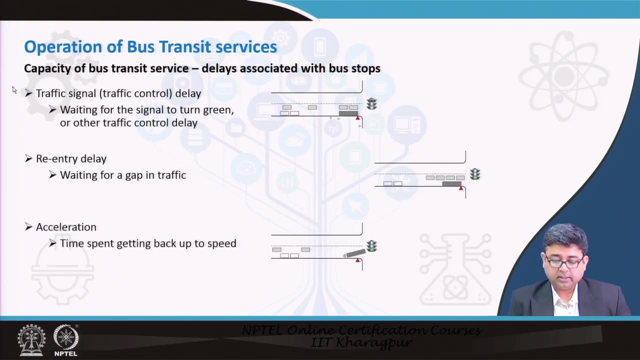 for the passengers to board and alight the bus. So all of this contributes to the delay associated at bus stops and these delays essentially then reduces the capacity of the bus transit system. ah, The other ah, the the other three ah situations are: ah delays caused due to traffic signals: right waiting at the traffic signal to turn. 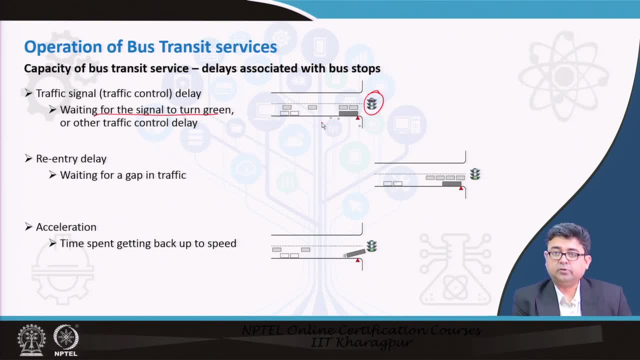 green or something or the other, even if you, ah, you may not have ah free, ah, free left turn in our situation, right, ah, the buses may not be able to turn free left, even though, ah, there is a, there is a ah, Ah, Left turn lane also may be, but ah, the signal said no turn on left, no turn on red, ah. similarly. 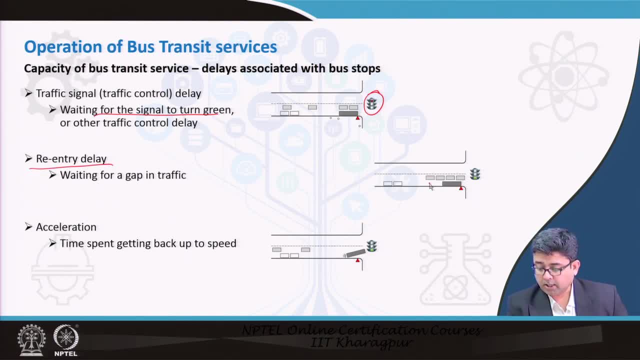 there may be re-entry delay. So if you already have entered into ah, the bus stop ah, but now there are other vehicles that are not allowing you to get back out, So there may be re-entry delay. and then there is some delay because of accelerating back from your stop. 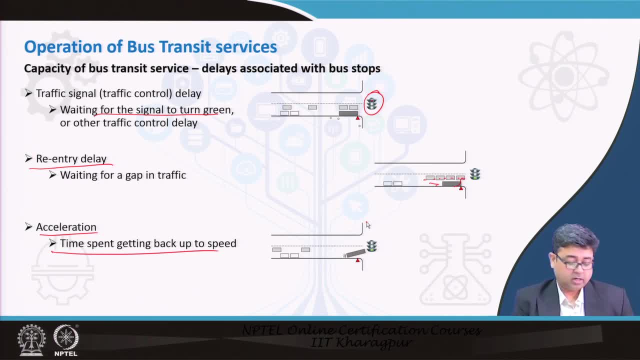 to the speed that you want to pick up. So all of these, all of these things cause delays to the ah Ah Bus service, are to cause delays to the one particular bus, which then can be accumulated into the entire service, and then that reduces the capacity of the bus system as a whole. 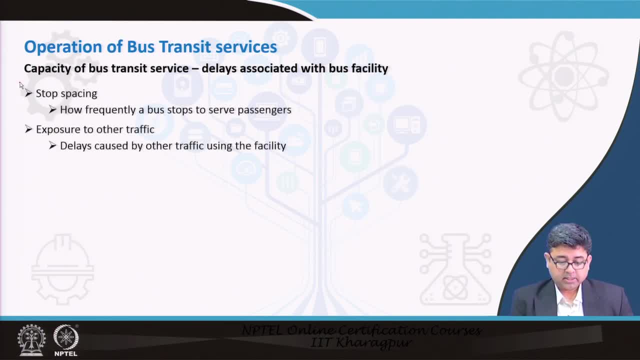 ah, stop spacing. Now, if you start looking at delays associated with the bus facilities, what are the different types of bus facilities? ah stops may be one type of facility. exposure to other traffic: ah On on ah. mixed traffic. ah, mixed traffic facility. if you are running your buses on a mixed traffic situation at 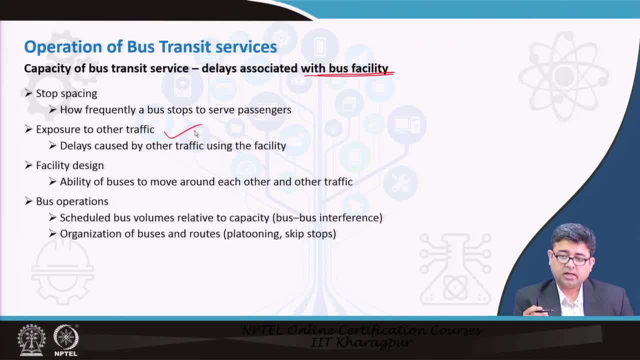 grade, then you are exposed to other kind of traffic which causes delay. We have told you if the spacing on one hand, if it is close to each other, you may maximize your person capacity, but then the bus has to stop every 20 meters, 30 meters. that reduces the speed. 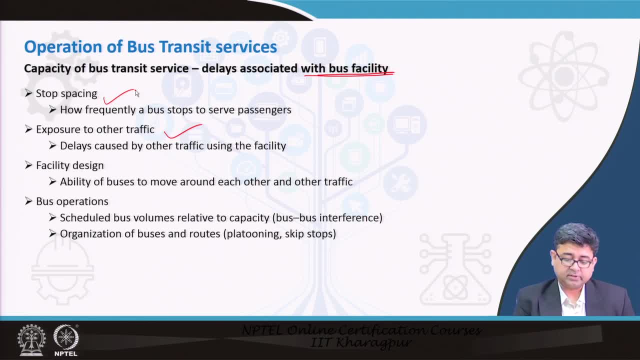 and that the increase, the delay and then reduces the capacity of the system as well. Facility design may be, the streets are do not provide enough turning radius at certain junctions, So the speeds of the buses have to be really slowed down or they may not be. 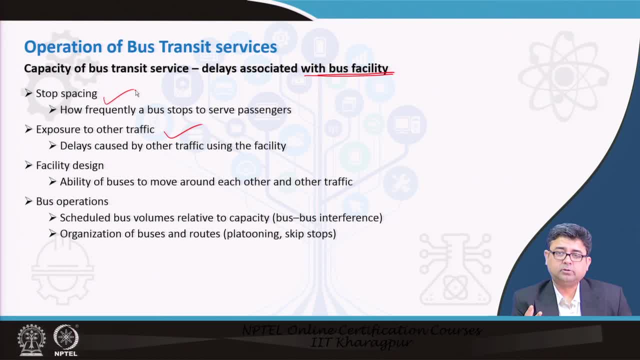 able to enter that route or that lane and hence has to go around, and that increases the travel time or reduces the capacity. again, operation factors that ah comes into play, whereas more and more ah due to ah, ah, due to congestion situations, there will be platooning: the 2 or 3 buses are bunched together and 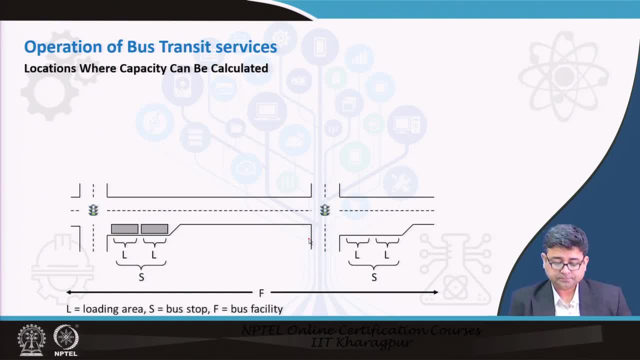 that causes again a reduction in the capacity. So where can? what are the places where capacity is calculated when it comes to a ah bus transit system? ah, it can be calculated at the loading areas of the bus berths right. ah, these are the loading areas usually. So you can capacity. 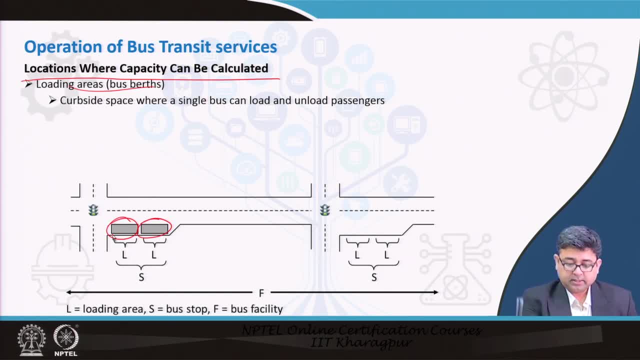 you can calculate the capacity of loading areas ah, that is, a curbside space where single bus can load or unload passengers- ah. you can ah measure the capacity of the bus stop ah together with the loading areas right. So if there are 2 loading areas in a bus stop, 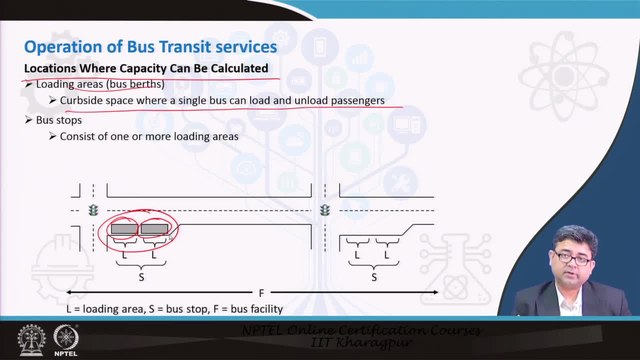 then the entire bus stop consists- ah, you can measure the capacity of the entire bus stop as well. And then, lastly, you can of course, ah, ah, ah, measure the capacity of the bus facilities which consists of one or more consecutive bus stops. So this is the entire facility. 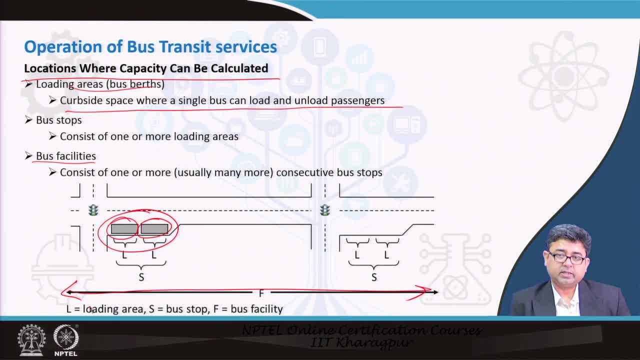 for which also you can conduct ah, or you can measure or estimate the ah capacity of your ah public transportation system. right, So it can. you can do it at a, at a, at a very micro level, at the, at the loading areas, you can do it at a meso level at the stop, or you can 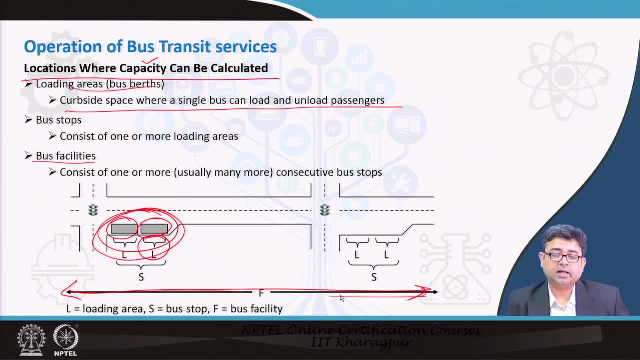 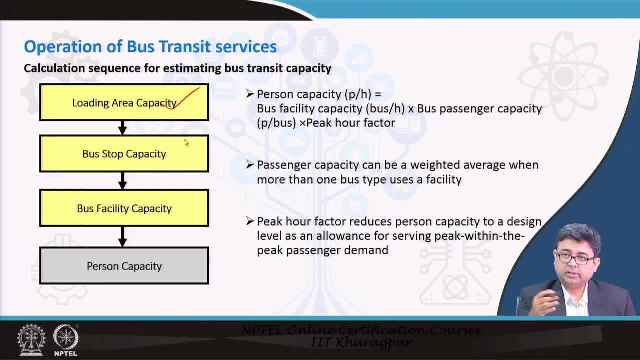 do it at a macro level. At the facility you can measure the capacity at 3 different levels. the loading lo limited 5, can control a bus stop through last DC food Crowd load capacity. So by knowing the load loading area, by loading, that is the lowest ah denominator, if you will. 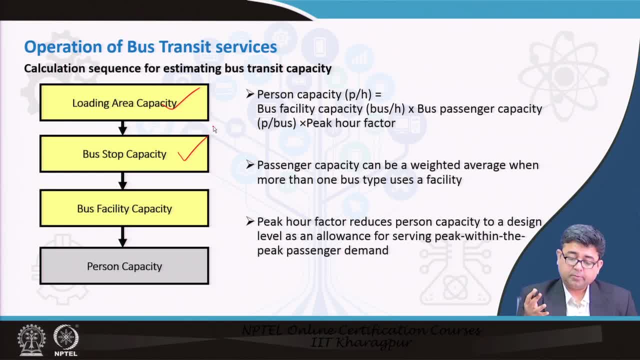 where you can calculate the capacity, can then aggregate it up to the bus stop, to the facility, and then you can convert it into person capacity. So the person capacity is nothing but the bus facility capacity times the bus passenger capacity times, a peak off factor There is. always a peak or factor. there is a peak or factor here. So in this situation the bus facility capacity is 0 and then the bridge capacity is 0. actually might be 90 degree plus development time, So that will be 50″ per person per bus and then a. 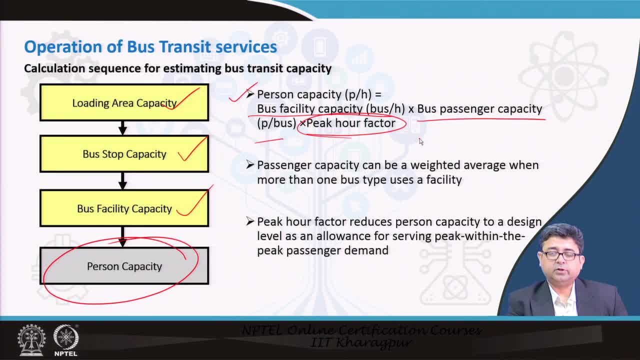 is always a peak hour factor because, remember, in the previous lecture, we told you that, ah, the ah bus, ah operations vary based on ah different hours of the day. ah, there may be peak hours and within peak hours, there may be peak periods as well. So there is always. 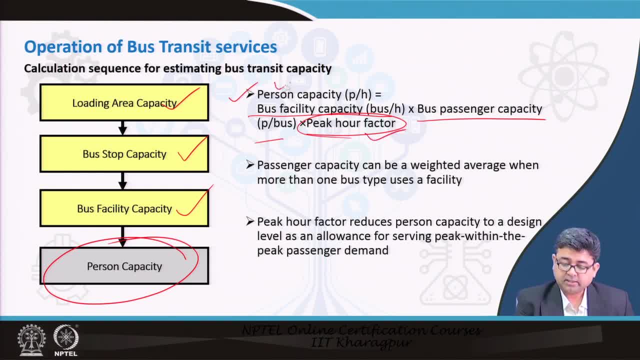 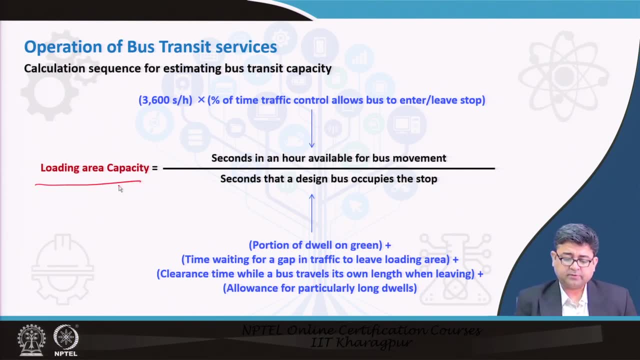 a peak hour factor that is factored in in order to understand what is the person capacity or the number of people per hour that your public transport service can move right. So there are simple ah formulas for understanding what are ah, how to measure or how to calculate. 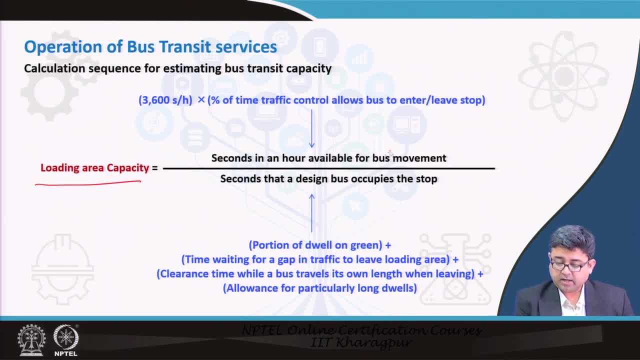 ah. load area capacity. It is the seconds in an hour available for bus movement, divided by seconds. that design bus occupies the stop. These are in the units. both are in the seconds unit, So it is a unit less ah. ah a measure. So what you all have to do is you have to. 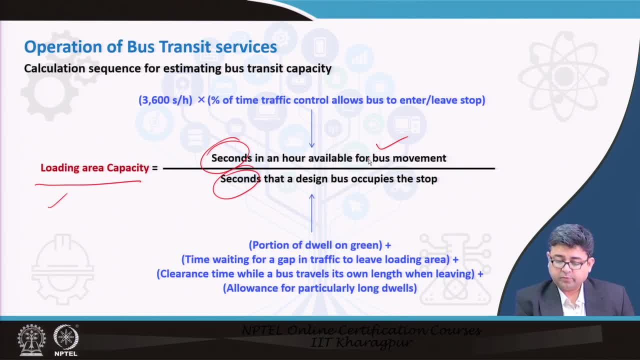 know how many seconds in an hour is it available for bus movement? That means there are 3600 seconds per hour. multiply that by the percentage of time ah, traffic control allows the bus to enter or leave that stop. So you have to do some manual calculations or you have to understand. you have to ah, wait, ah, be at. 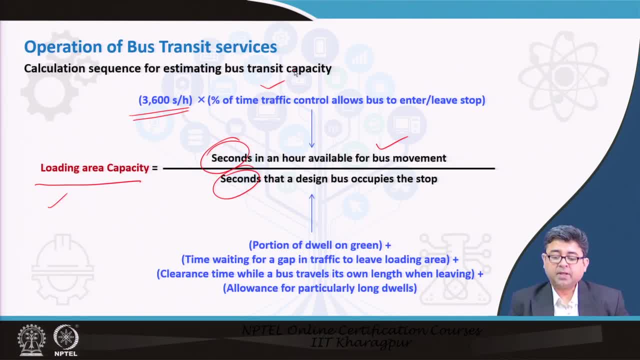 a bus stop, a bus station and figure out how much time, ah, how, what percentage of time does? does traffic control? traffic control meaning the traffic environment around around that bus stop. So the bus travels its own length while leaving. So when the bus is leaving out of a bus bay. 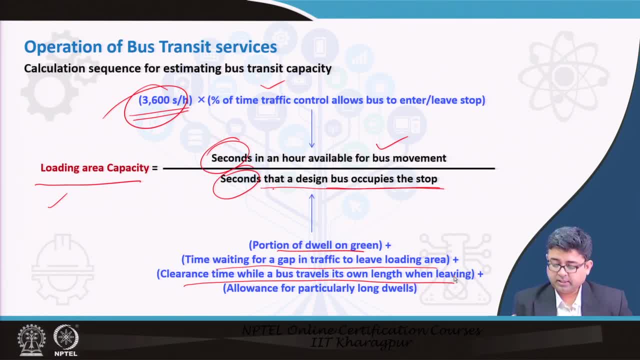 its entire length. it has to cross the entire length. So that is the ah ah clearance time needed and allowance for particularly long dwells. Sometimes ah, the dwell times are longer if there are large number of passengers loading from that ah ah, loading, embarking or disembarking. 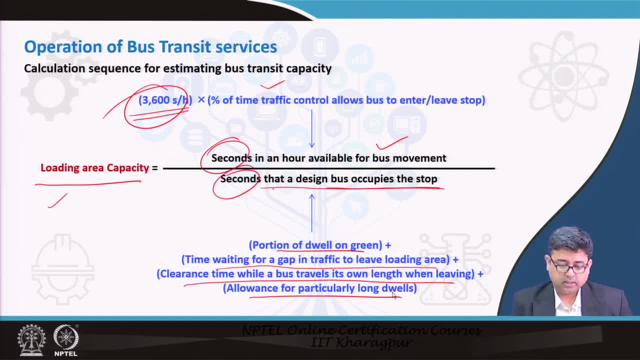 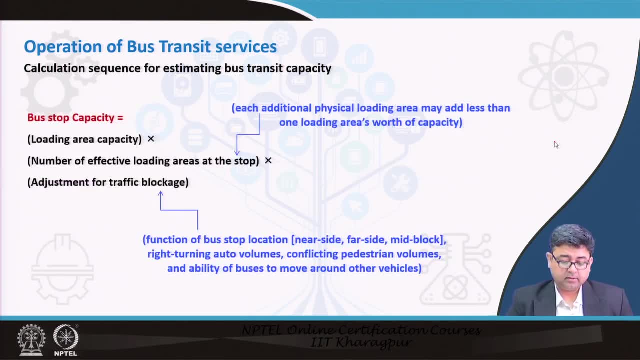 or boarding from that ah, ah loading area or that stop Right. So that is a simple, simple enough ah, ah, ah, ah ratio to find out Similarly, ah bus stop capacity now can be now ah, calculated by multiplying the loading area capacity that you have already figured out by by the number of effective loading areas at that stop right. 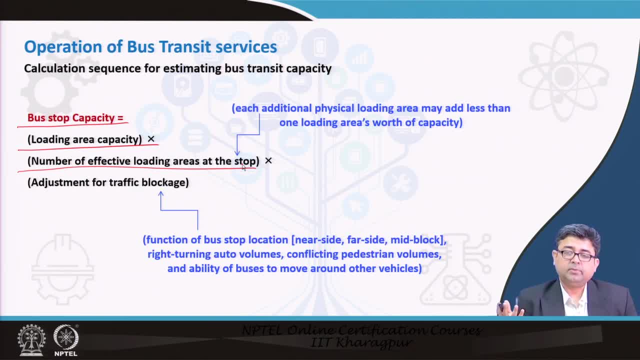 There may be two loading areas, but one may not be available because of, ah ah, encroachment or whatever it is some other reason, parking vehicles parked on there. So, or even this, ah, the existing ah ah bus may not have docked at the, may not have stopped at the right. 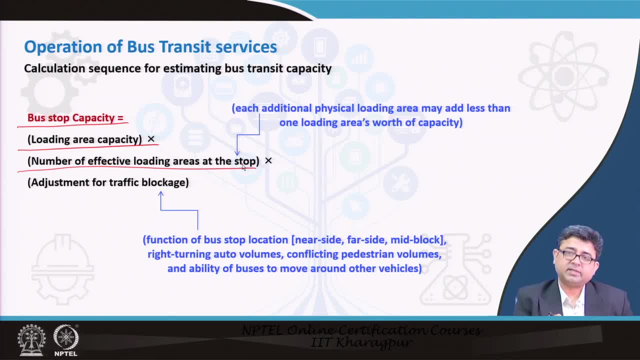 position. So it may have taken up ah, both the spaces ah and the other way. other bus is not unable to come inside this ah loading area. So there may be, but so that is why you have to calculate the number of effective loading areas and not just the number of loading. 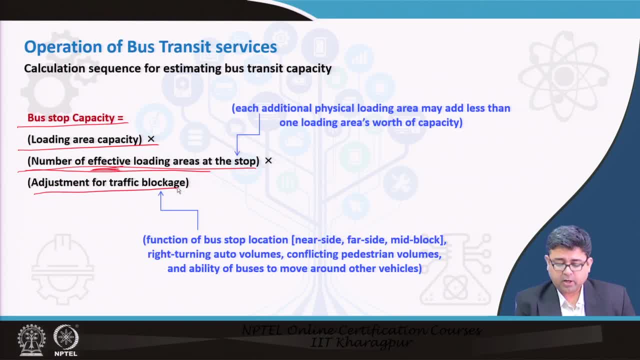 areas at that stop, and the adjustment factor for traffic blockage, which is a function of the bus stop location. ah if it is blocked by ah parked vehicles, for example, for right turning or left turning volumes. ah if there is conflicting pedestrian volumes. So there are, there are different adjustment factors. these are standard factors that have 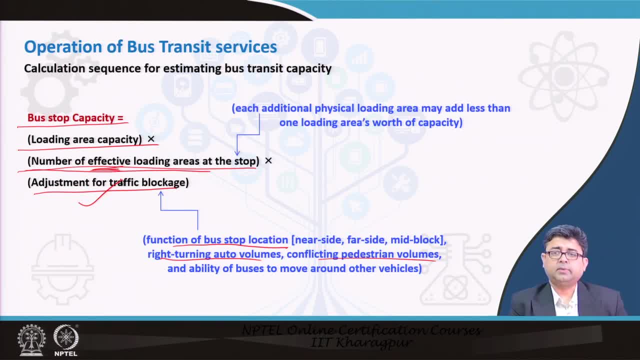 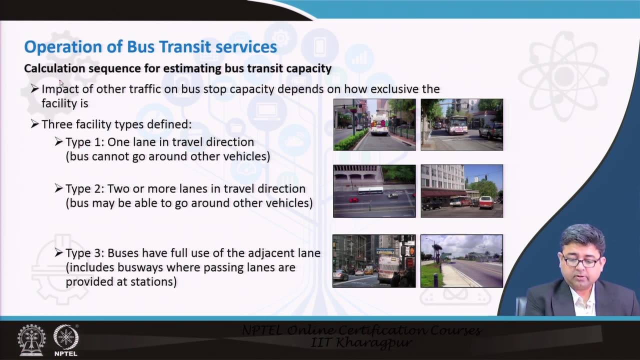 already been developed ah in many based on many operation, many operating conditions ah. you may adopt that for your ah situation or you may develop your own factors ah based on your ah um local traffic conditions as well. So basically, ah then for calculating ah and estimating the bus transit capacity you have. 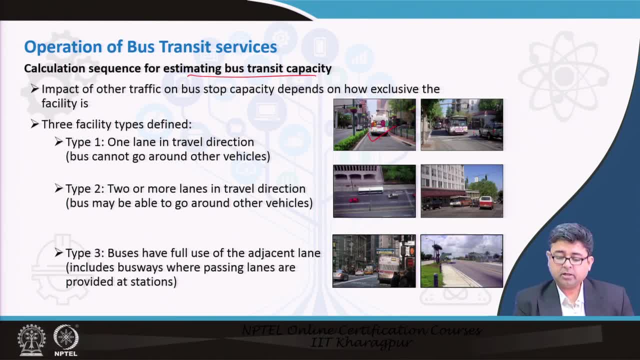 to know, ah, what type of facility your bus is running on. ah, is it a one lane? ah, one lane, one direction, ah. unidirectional facility where the bus cannot overtake any other vehicle, So if there is some vehicle in front of it it cannot overtake. that limits the capacity. 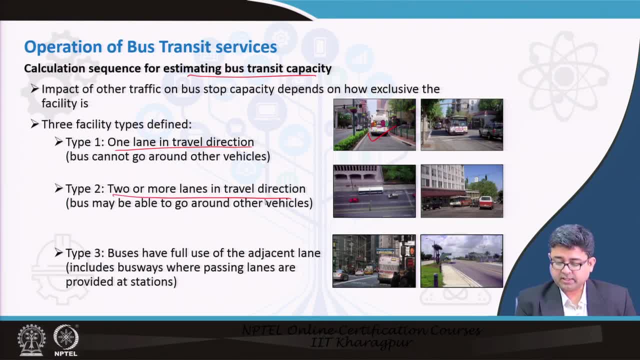 of the bus ah of your system. If there are two or more lanes in the traffic direction, ah, then ah your bus may be able to overtake and ah access the bus stop, Or ah do a turning movement or whatever that allows it to ah ah move faster in the traffic. 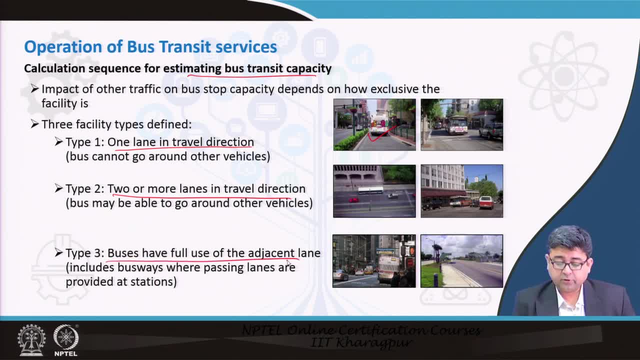 stream or ah type 3, where the buses have full use of the adjacent lane, including bus bus ways. So you have ah, ah dedicated right of way for the buses to move. So that type of system also ah is the best for when it comes to ah having good capacity for the buses. 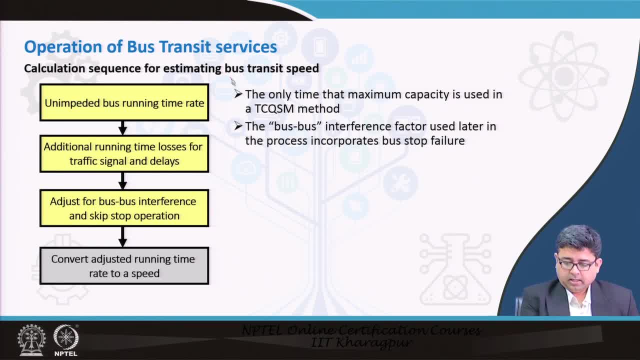 A given period of time. right based on the speed limit. ah, you can calculate the ah bus that you can assume that this might be the rate of buses that is going through that segment. ah, then you ah start to account for different types of losses. Now, then you try additional. 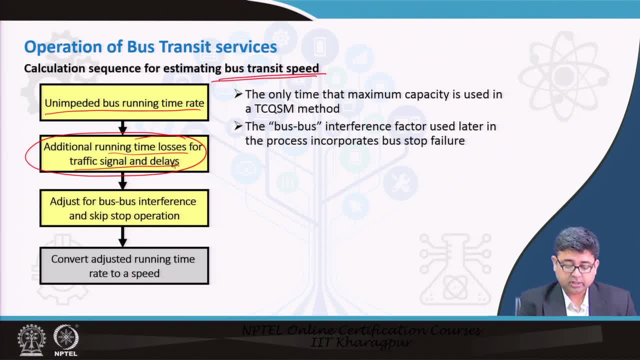 running losses for traffic signals and delays. Now you say, add those losses, adjust for bus, bus interference and skip stop operation. ah, when this bus bunching happening. ah, that reduces the bus speed. you take into that, that into account. after all that, then you convert the adjusted running. 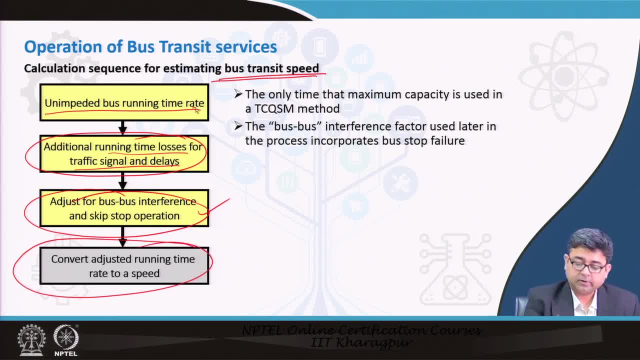 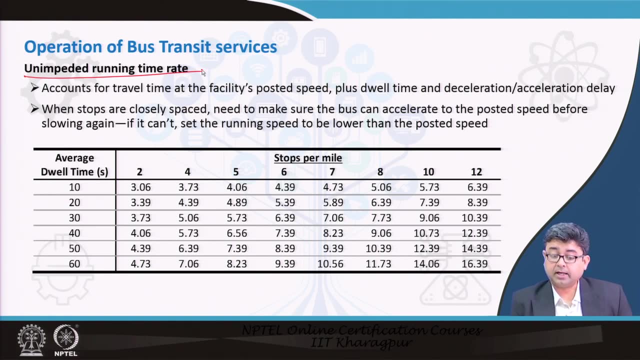 time rate to a speed. Then you convert this, use all these last times and then finally convert them into a speed. So let us look at how unimpeded running- what do you mean by unimpeded running time rate accounts for travel time at a facilities posted speed plus. 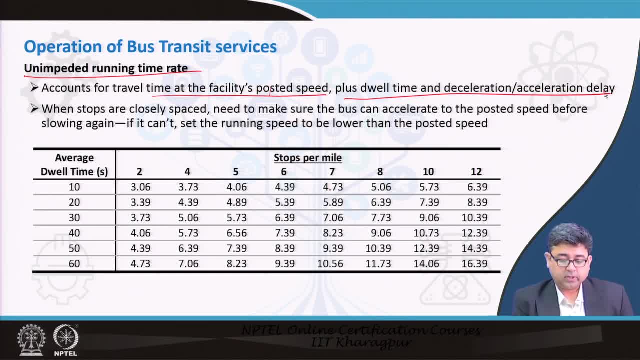 dwell time and acceleration deceleration delay, right? ah. So what, whenever the- whatever the posted speed is plus your dwell time and acceleration deceleration delay will give you the unimpeded time rate when stops are too closely spaced? ah, need to make sure that. 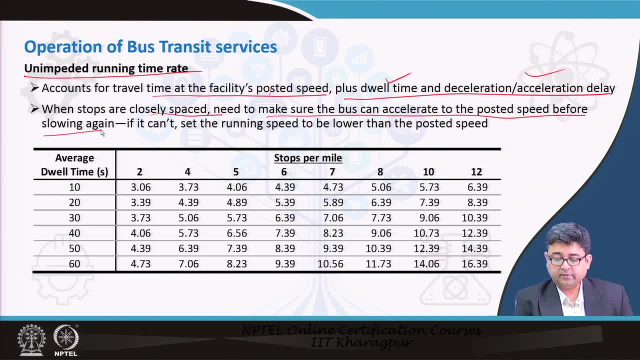 the bus can accelerate to the posted speed before slowing again. if it cannot, then you set the running speed at a lower than the sports. If the if the two stops are too close to each other, then there might be a situation that the Bus Bus. 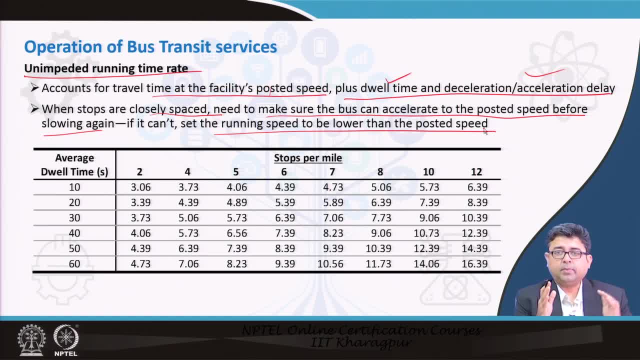 Bus may be able to reach 60 kilometers per hour top speed, but since it is the next, the next stop is only ah 500 meters away. it cannot get back. it cannot accelerate up to maximum speed, it can only accelerate up to maybe 20. 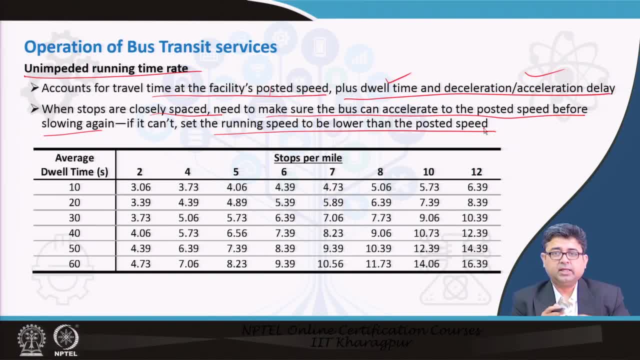 kilometers per hour, and then it has to start decelerating again. So then the speed that it reaches is never its maximum speed. So you have to then, ah, let it run at a lower speed than the posted speed limit as well. So these are standard ah numbers, that are: 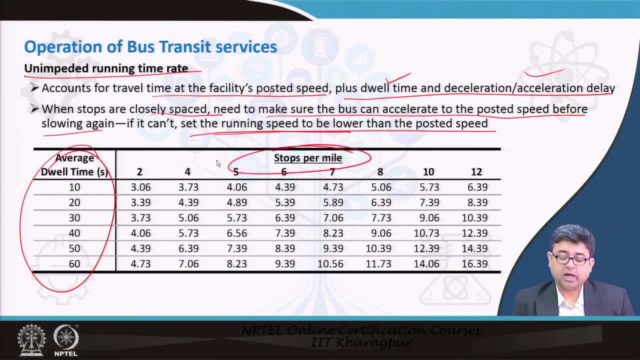 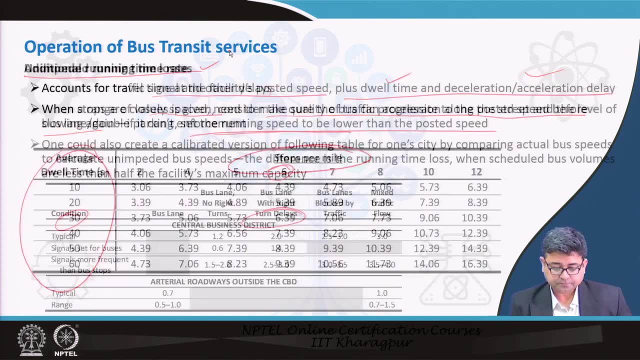 used for average dwell times and how many stops per mile if you have. So if if, for example, you have 6 stops per mile and your average dwell time is 10 seconds, So the this is what you are going to have as your unimpeded running time rate. ah. Additional running losses. 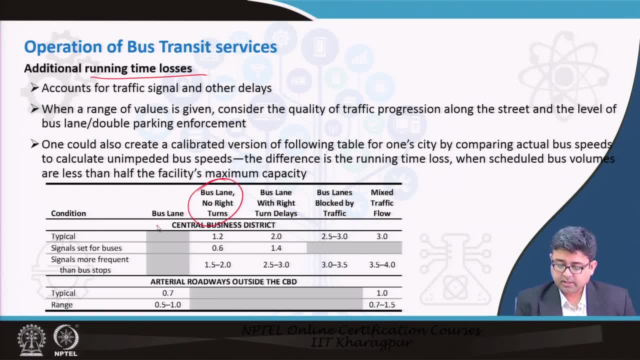 also ah running losses because of right turn lanes, because of mixed traffic flow. So there are different ah in for different types of land uses. For example, on arterial roads outside the CBD and in the central business district you have different ah. such figures that have been calculated mostly in the western countries. 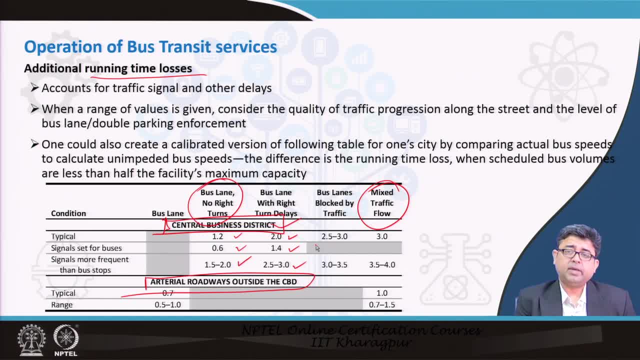 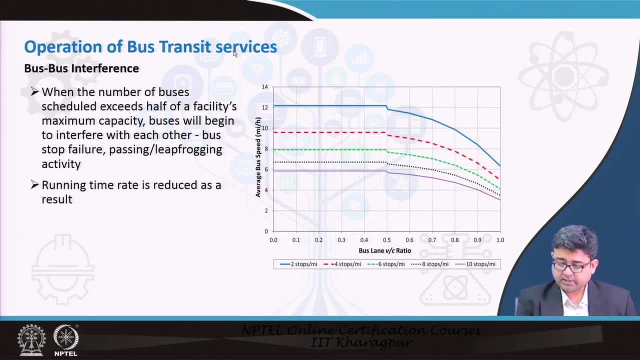 but ah, you get the idea of how to measure this and what may cause the delay, and you can ah carry out similar ah running losses as a running time losses for your city public transportation network as well. Ah, bus bus interference, as I was saying. ah, if there are ah. 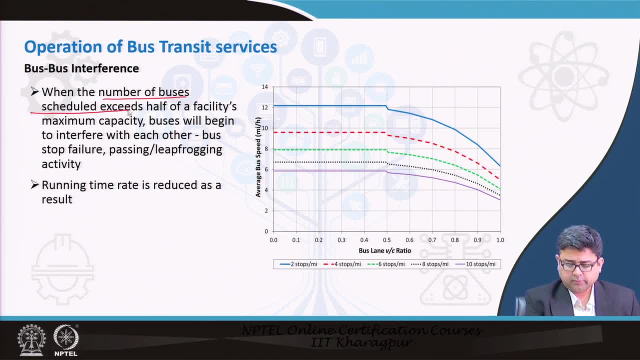 So when the number of buses ah schedule, ah schedule, or when the number of buses schedule exceeds half of the facilities maximum capacity, So if it is exceeds half of the facilities maximum capacity, buses will begin to interfere with each other. So, bus bus failure, ah passing. 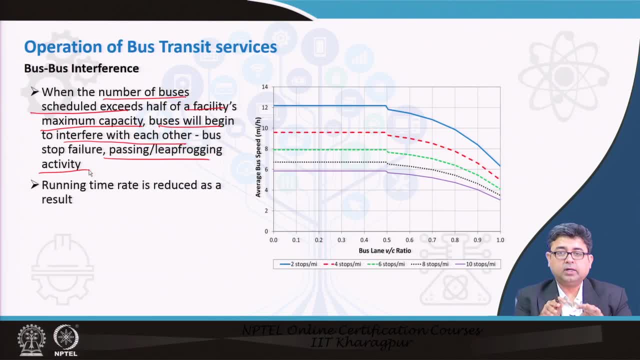 leapfrogging activity. So when you see two buses- ah trying to race against each other, right, that is when you know that your bus bus transport network is not functioning well, because they should not be competing against each other. They should be helping ah or working ah ah in parallel to each other, So that the efficiency. 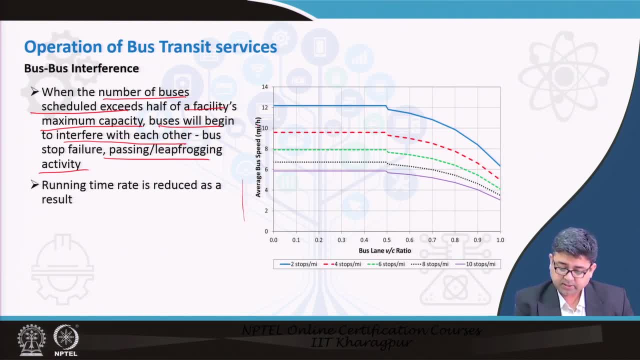 is increased. So what happens to the bus speed? So you see the bus speed average bus speed goes, starts going down when the ah bus lane ah V by C ratio starts going up. right, There are more number of buses ah than the capacity that ah it can hold ah in that facility. 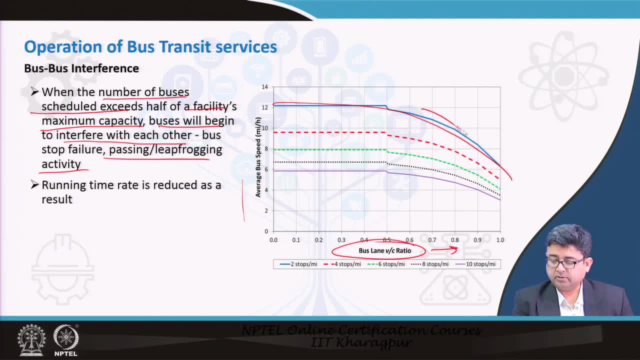 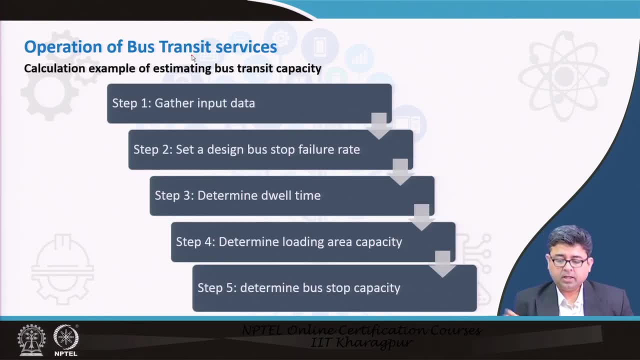 So as that keeps on increasing, your bus speeds goes on reducing. So that is what we are discussing. So you never ah have too much ah bus bunching going on in your system. So this is a generic ah ah steps that are usually calculated, ah usually done in order. 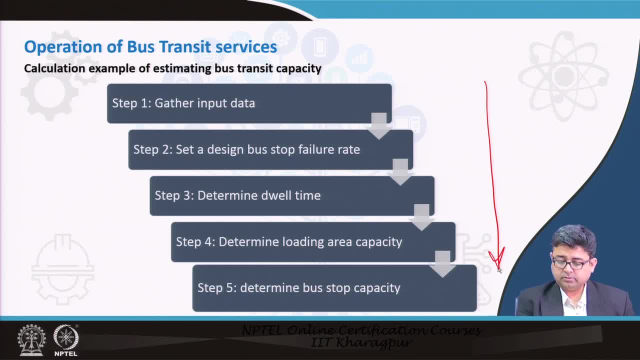 to estimate the bus transit capacity? ah You, you design all you ah. you get all the background data- socio economic data, ah demographic data- from your, of your city. You set a design bus stop failure rate right ah 17. Then against that ah design rate, you start determining the dwell time, determine the. 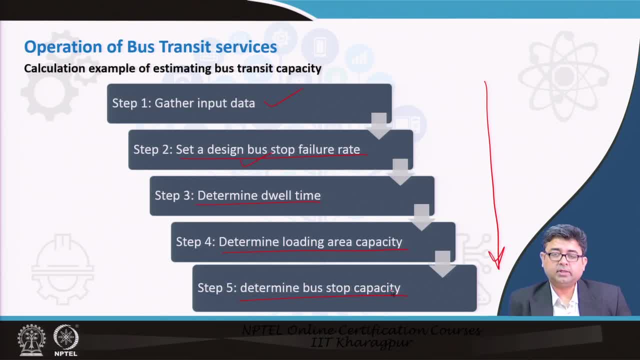 loading area capacity and then determine the bus stop capacity. ah. You, you have understood that the loading area is the ah lowest denominator, then it is the bus stop capacity and then it is the bus facility capacity. So here we are only ah stopping at the bus stop capacity. 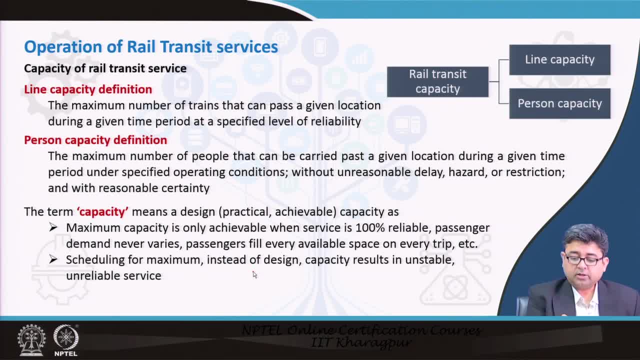 level. So next, if we start looking at the ah, ah, rail transit services- ah, their capacity calculations are also. the principles are very similar to a bus transit capacity, but there are few other factors that ah come into play when you are trying to calculate rail transit capacity. 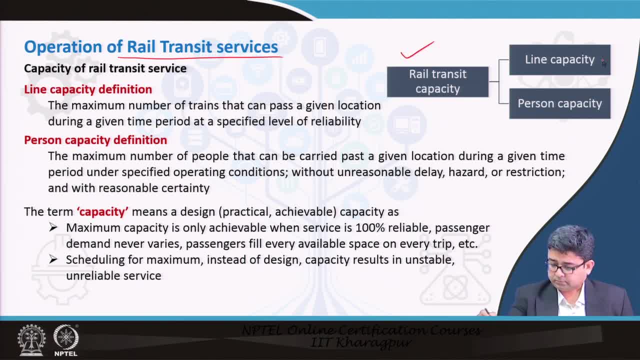 ah, Like you say here, like we look at here, a rail transit capacity depends upon. there are two different things that we talk about. it is either the line capacity or, again, the person capacity. So you know how to measure. we have person capacity, ah in terms of ah, when we 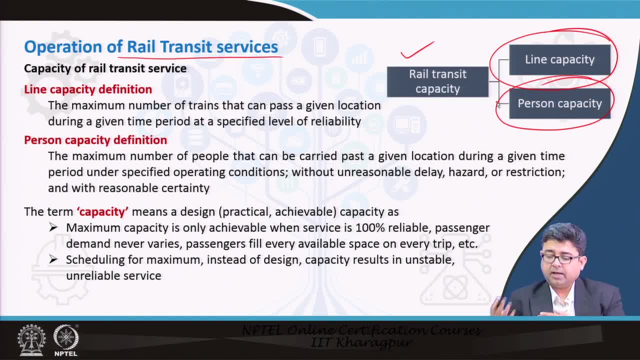 talked about ah bus bus transportation systems, ah, But we never talked about line capacity in ah in bus transports, ah in bus transport systems. So let us look at what is line capacity here. line capacity is the number of trains that can pass a given location ah during a given time period at a specified level of reliability. 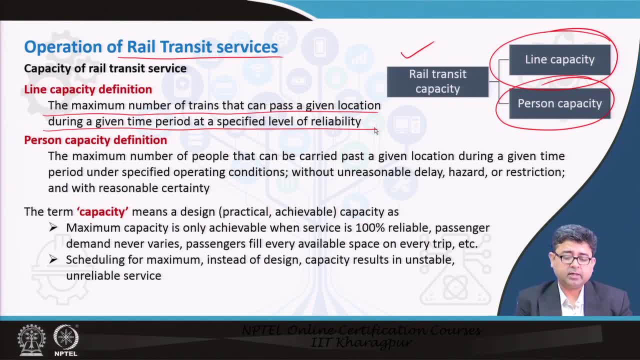 So you see that the definitions are also very much similar: ah. there we had ah bus capacity or vehicle capacity. here we have line capacity. ah, person capacity is a similar to ah. what we have ah in the bus transport. Ah 17 0. 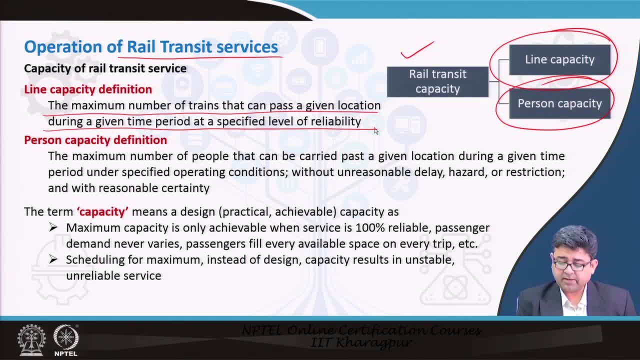 arena as well. ah. Again, here also we have reliability, ah. So maximum capacity is only achievable when service is 100 percent reliable. passenger demand never varies, So this was the situation for bus transport as well. So when you talk about bus and rail transport, 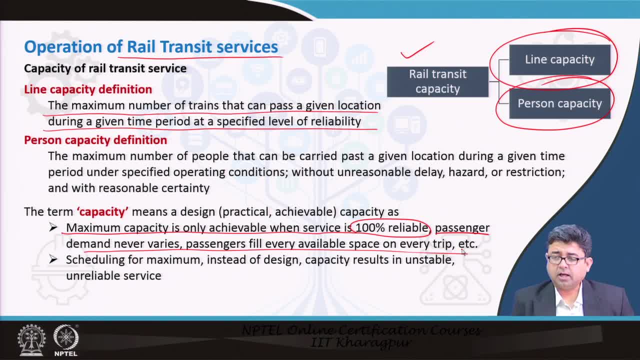 the basics are very similar. ah, The basics are very similar ah when it comes to measuring the capacity. there are few other elements that we look at ah in rail which are different from bus, ah, and that will give you an idea of it. So, ah again, dwell time is very similar. 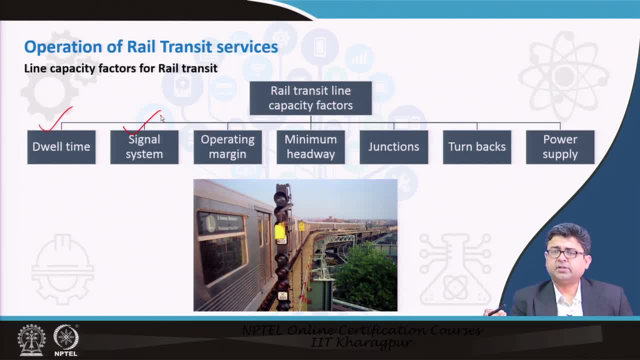 ah signal system plays a role, important role ah, Even for bus transport. the signaling on the urban roads plays an important role, but in for rails they have dedicated signals ah, which also play a role in ah understanding the capacity of the rail transport system. ah. Operating margin is something that plays and we will see what that is ah headway like. 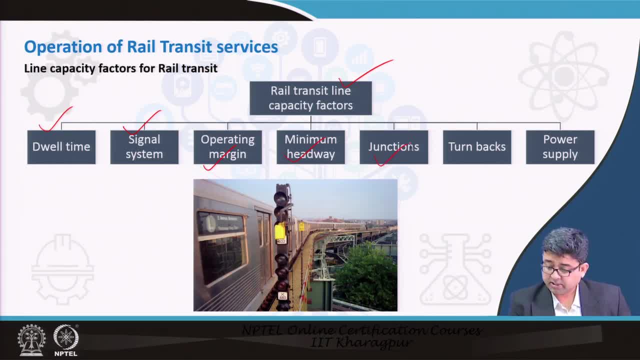 we have looked at So even in the bus, in bus situation. ah junctions here play a role. turn backs is something that ah buses do not have, So we will take a look at that. and also power supply, which again buses- ah buses do not have to be plugged in unless they are now new electric buses. that. 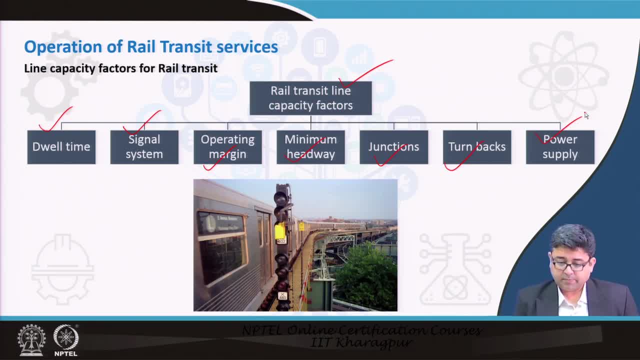 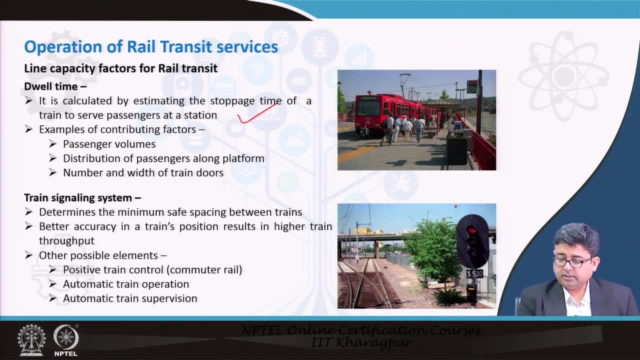 are coming into play, So they will be affected by power supply. So dwell time: we already know it is calculated: a ah the the amount of time that a transit vehicle waits at a stop and to allow the passengers to ah board or disembark. 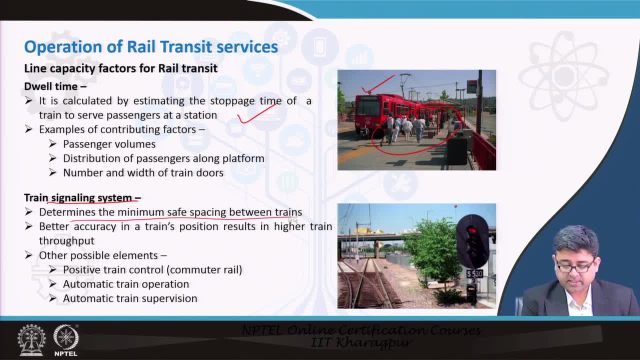 Train signaling system. so this determines the minimum safe spacing between trains. ah. So better accuracy in a trains position results in a higher train throughput. right Now, train signaling systems are very, very important because ah not only from the capacity point of view but also from the safety point of view ah. So these ah possible elements ah. 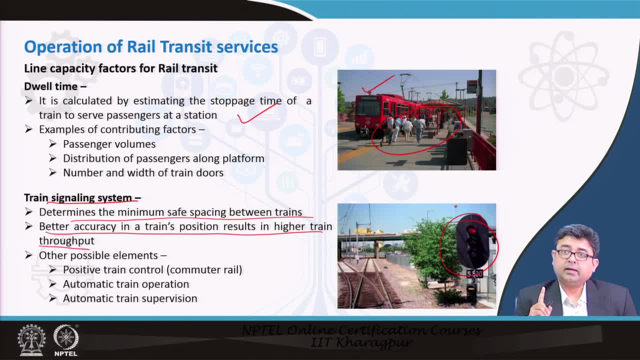 these kind of signaling systems ah. So when they are ah trying to improve the capacity, they will, however, always keep in mind ah that ah the signals will not ah interfere ah with the safety of the system ah in order to increase capacity. So capacity will always be ah secondary, and safety will always be. 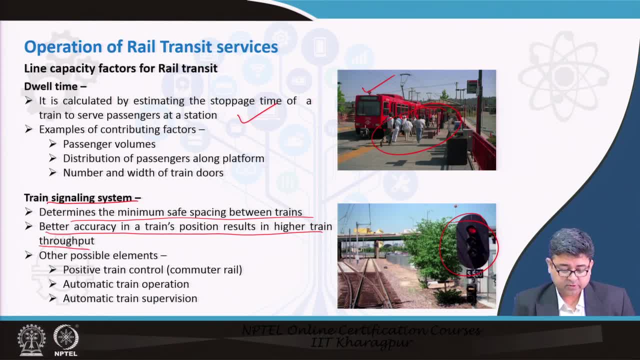 primary when it comes to ah, ah train signaling systems. Although you would want to have a signals give a lot of ah- minimum red time and more green time and ah green, more green time more frequently So that more trains can come. but ah, that may impede the safety. 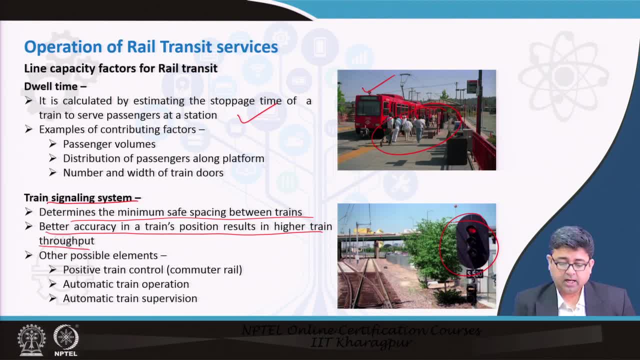 of the train systems, right ah. So that is something ah to keep in mind when you are trying to ah design your ah or train services, or train public ah, public transport services in your urban area. This, I am not getting into intercity rail, yet ah, This is just ah, we take this into consideration. ah, ah for Metro Rail services. 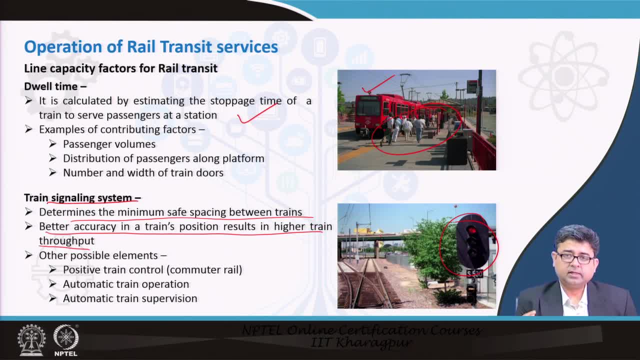 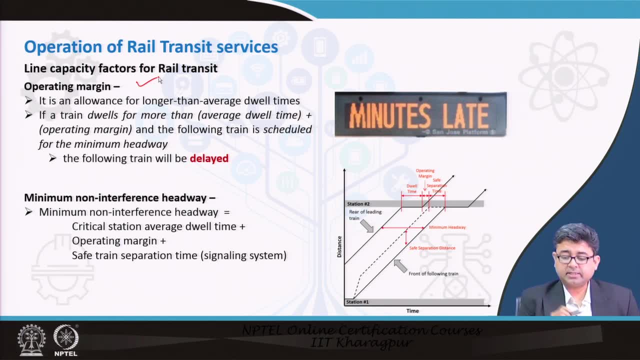 for example, Ah, When train lane integrates, this will stay in the City rail system or may be light rail services that may be available in your city Operating margin. now, this is something that rails always, rail systems always, worry about. So it is. this is an allowance for longer than average dwell times. 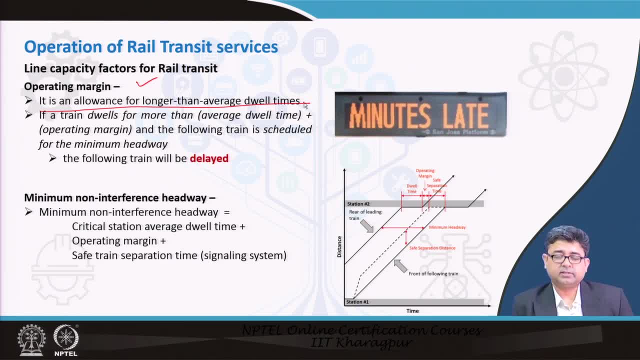 So usually what happens is sometimes the trains wait at a station for a longer period of time because there are multiple cars in a train system and to load and unload passengers it may take longer than average dwell times. So if a train dwells more than the average dwell time plus the operating margin and the 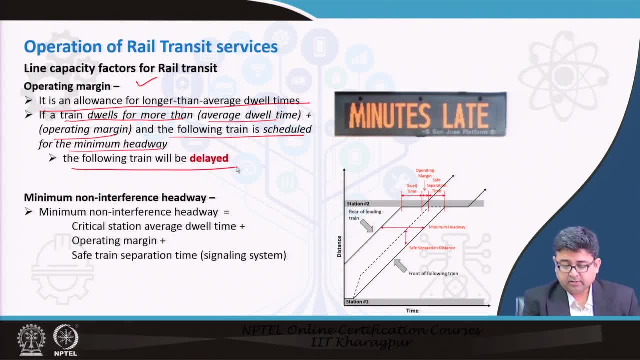 following train is scheduled with the minimum headway, then the next train will be delayed, right? So this, there is always this operating margin that is given to all the trains, So all the train services, to the each of the train lines that you have, this buffer. 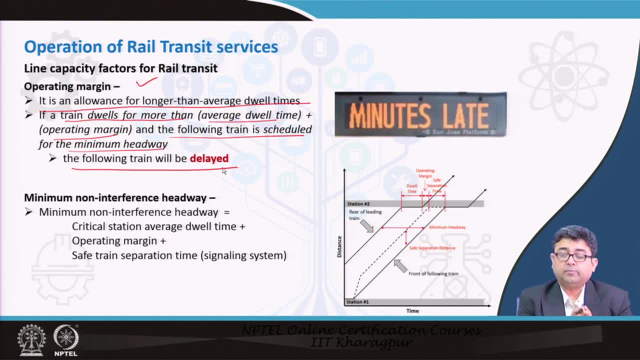 So this is all. the operating margin can be looked at from the point of view of a buffer, that you have this buffer time, that if you want to wait in a station for 2 more seconds, you can do so. however, you have to leave within the next half a second because otherwise, 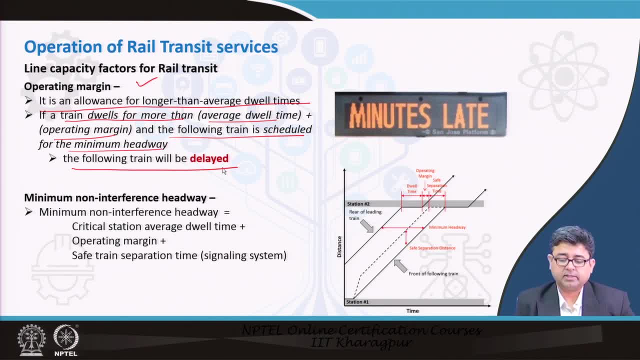 if you do not, if you, if you cross that threshold, if you cross that buffer margin, then the next, the train that is following you, might be delayed. So operating margin is sometimes, always, is always kept in mind very, very carefully when you are actually calculating how much dwell time each train should get at a station. 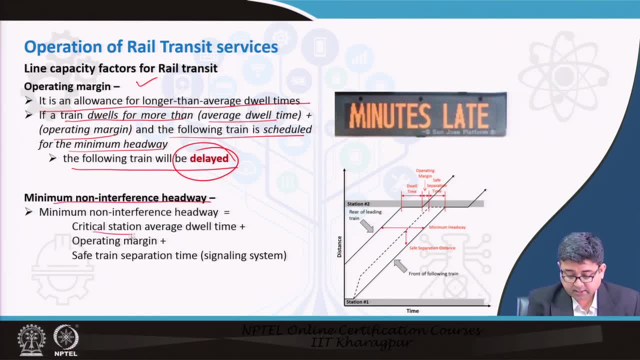 Minimum non-interference headway is equal to the critical station dwell average dwell time plus the operating margin, plus the safe strain, safe train separating time. Again, there is always a minimum headway. So minimum headway that has to be kept in case of bus transit. we we notice that we. 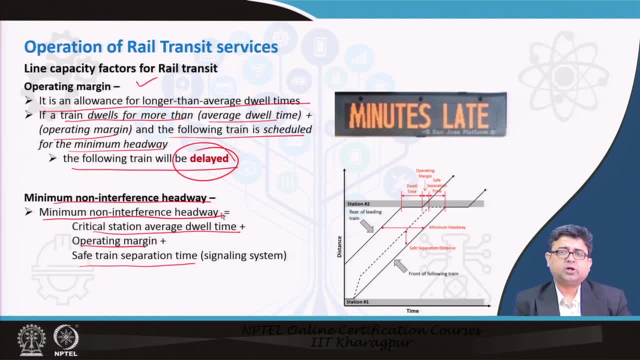 always try to minimize the headway as much as possible because it is easier in the case of buses to control the headway. but when you are on rails and when you are on tracks, you have to be, you have to maintain a minimum headway. you and you should not tinker with. 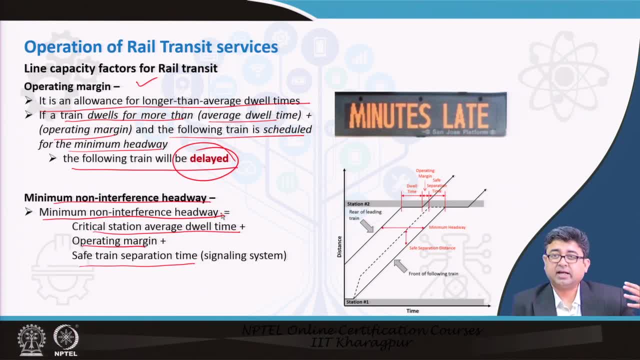 that minimum headway, because then, because the trains are usually at higher speeds, then it becomes very difficult for you to Decelerate at time, at the given time, and it may cause a collision with the train ahead of you. So always maintain a minimum headway and keep that in mind even when you are designing. 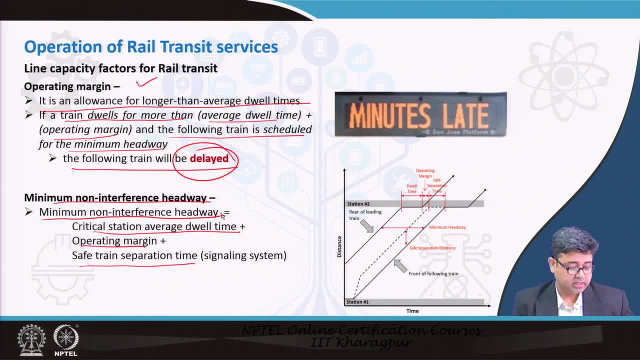 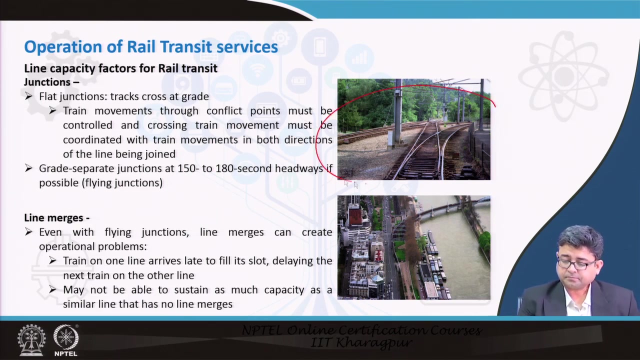 for maximum, maximum capacity, right capacity. remember again: capacity should not come as a in come in the way of lower safety. higher capacity should never come in the way of lowering safety. Ah, an important thing in in in case of trains, are these junctions right? These are. the picture, of course, is of a intercity rail ah system. but even in metro rails and 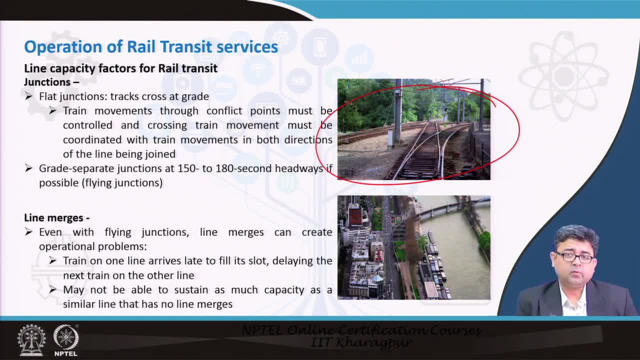 all you would have seen ah that there are certain junction areas where the trains have to turn around, or there are ah, multiple ah train lines, metro lines, that ah combine at one kind of rail station, So that becomes a junction. So what happens is that the tracks cross. 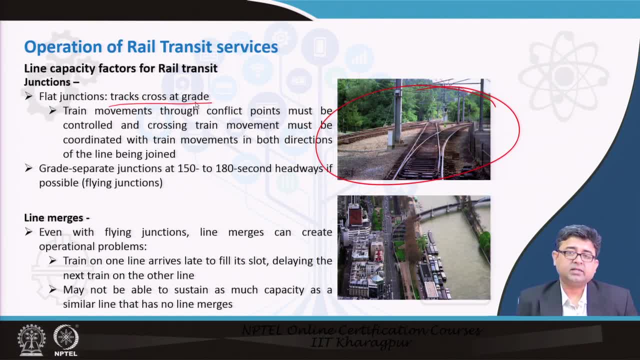 at grade. So when the track starts crossing at grade, that is, when at these junctions there is some delay that is incurred for to the movement of the trains, then the train movements through conflict points must be controlled and the train crossing movement must be coordinated. 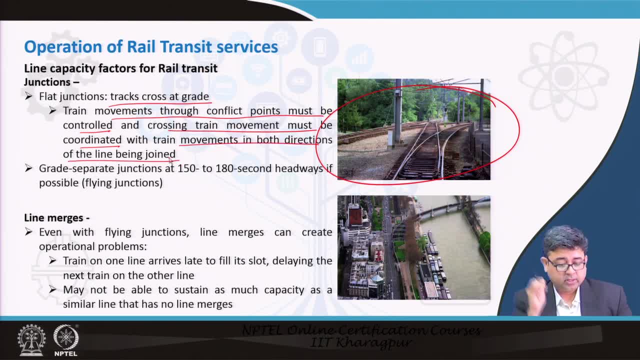 with train movements in both directions of the line being joined. So always 150 to 180 second headways, if possible, are given at grade separated junctions. So again, this adds to your delay and has to be taken into consideration when you are calculating. 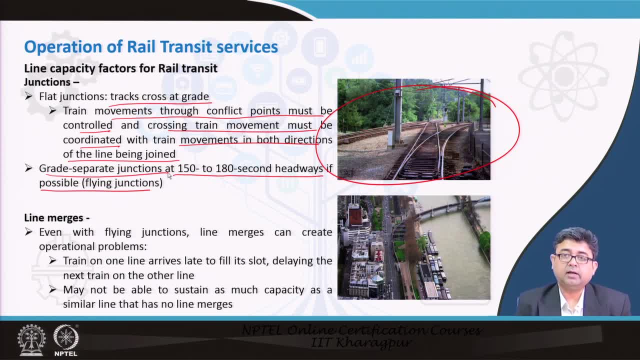 your, your headways as well as your capacities, Then there may be, similarly, there may be line merges at, at, at, at junctions where train on one one line arrives late, So it is so to fill it slot, delaying the next train on the ah. So, if, if, if, usually these have ah right. 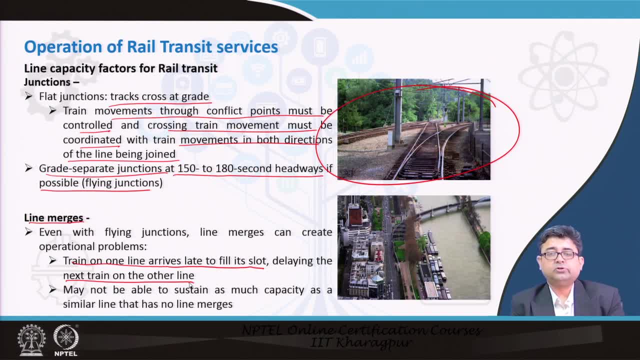 of ways right. So right of ways does 2 things. right of ways allows you, ah, ah, no interference with the other traffic, So you can, ah, you can, provide reliable travel times. but if anything goes wrong, ah, you have your dedicated right of way, So you cannot fix it very quickly. 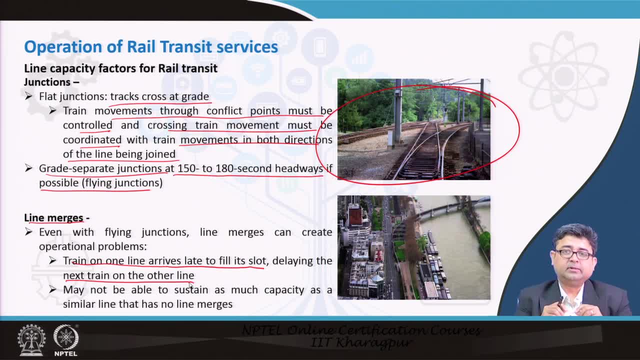 So smaller delays- try ah- adds up to making a large delay, So you cannot fix it very quickly, So you can add a larger delay as well. So ah, right of ways, ah, dedicated right of way, always ah- is something that has both advantages and disadvantages. 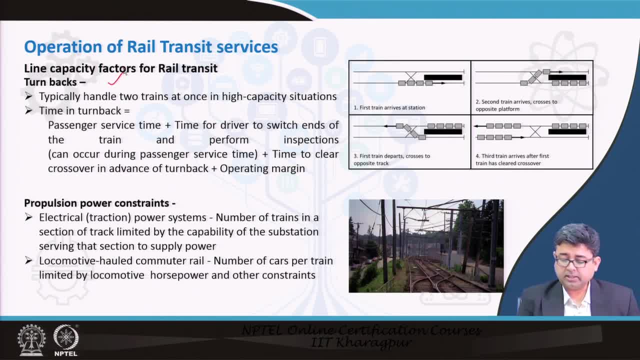 Ah, turnbacks ah. these are usually provided ah for ah at at railway stations ah, so that typically that can handle 2 trains at once in high capacity stations, Ah. so you see, if the, if the first train arrives and goes on this type of ah, this side of the stage. 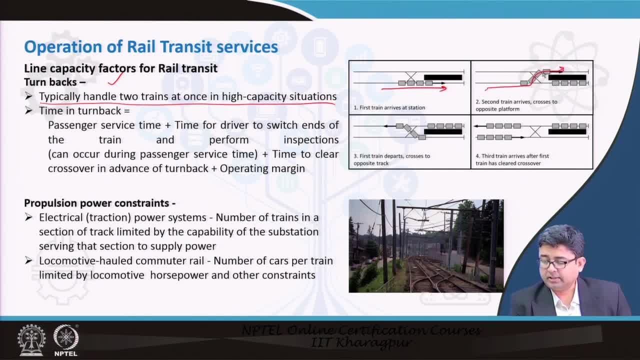 platform, the second train arriving can go at the other side ah, and that is why you provide this kind of a ah railway crossing ah, or which are called ah turn backs ah, and then if this station, ah, if this the train which came here had to had to go back, then it can again ah depart. 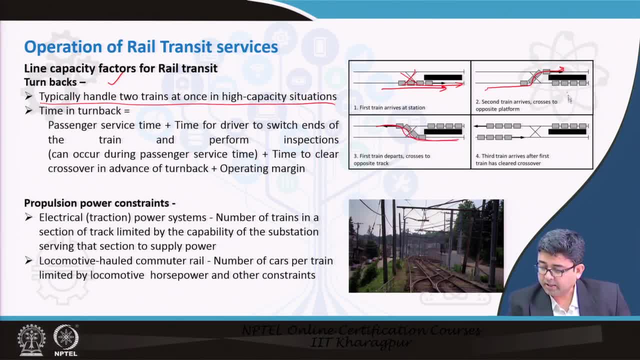 from ah that station, independent of ah, independent of this train which is now sitting at this platform, and another new train can come in and use this platform. so these turn backs are, ah, very, very important, ah, ah, ah, feature of ah of any rail transit systems, and they 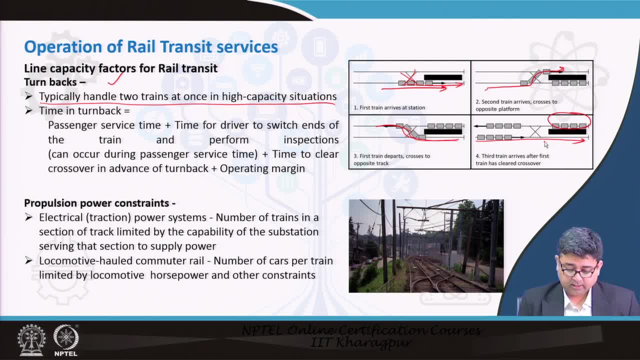 help improve the capacity of the train, ah of the ah transit train transit systems. and of course, then you have your power constraints: ah, electrical, ah traction power systems, locomotive halt, commuter rail. so, ah, this is more, ah ah, the number of cars per train limited by the. 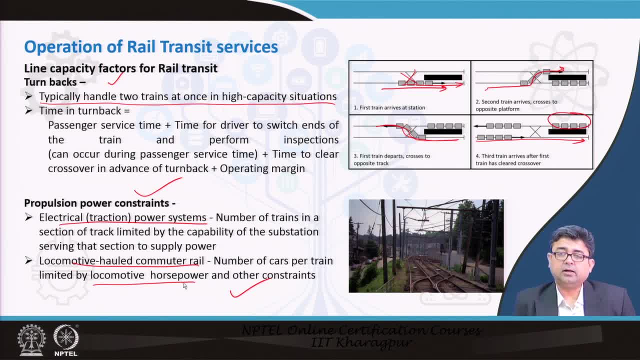 locomotive halt commuter rail. so this is more ah ah. the number of cars per train, limited based on the force power. ah, this is ah when it comes to, ah, you know ah, long distance or regional railway. ah, whereas ah h, electric traction power systems are more of your ah. 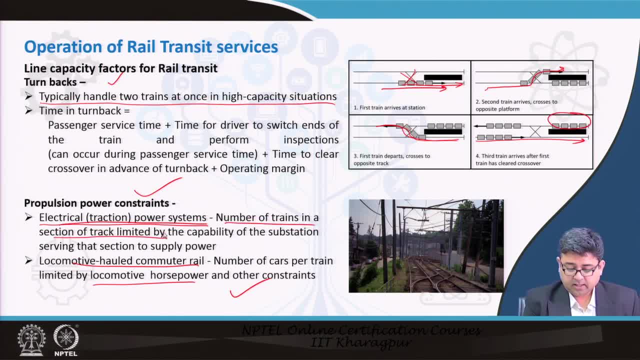 metro rails. ah number of trains in a section of the track may be limited by the capability of the substation serving that section that supplies the power right. so you have to keep in account ah, take into account the actual ah substation capacity that you are utilizing. 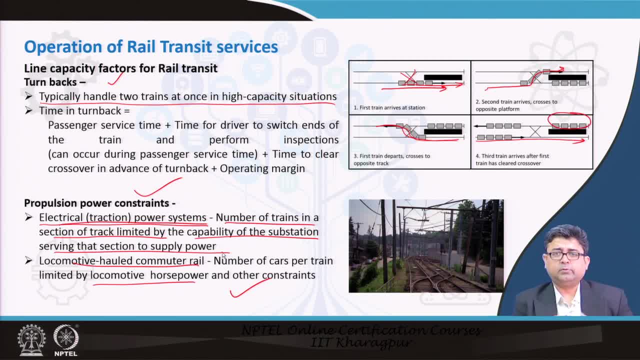 ah for your trains. So when people they are Ya, when people say that, why do not you add another metro rail, another car to the metro rail that arrives during peak hour? So usually we do not realize that that another car will another car, or bogie, for example, will need additional power and if we are already running at maximum, 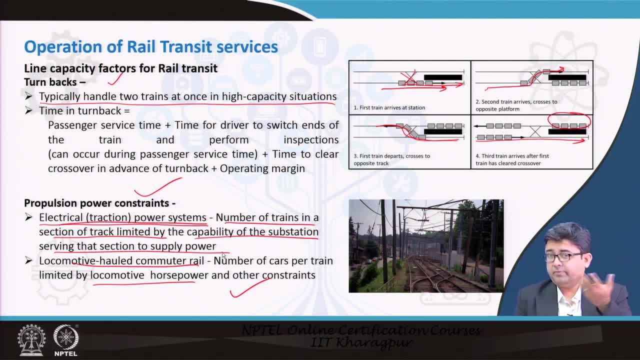 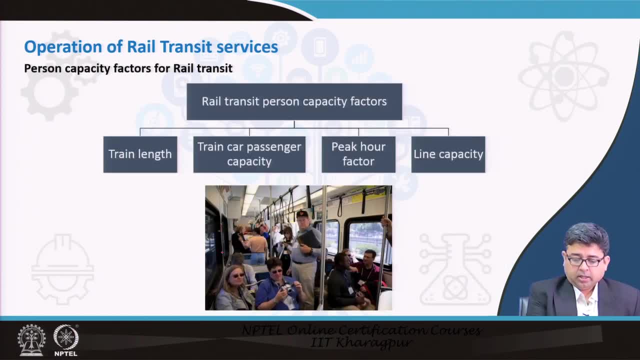 power from the substation from which we are drawing power, then we may not be able to add another car or a bogie to the rail. So what are the percent capacity factors for rail transit? Again, if you want to calculate percent capacity, the train length, of course. 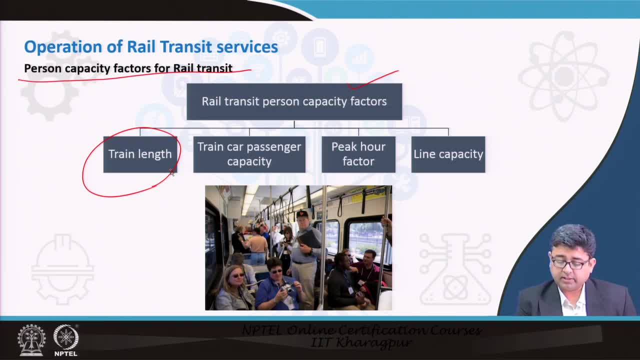 the number of bogies that you have, number of cars that you have in the train. the train car passenger capacity each car, how many sittings are there? you are allowed a few standing passengers to measure the capacity. then you will have always have a peak hour. 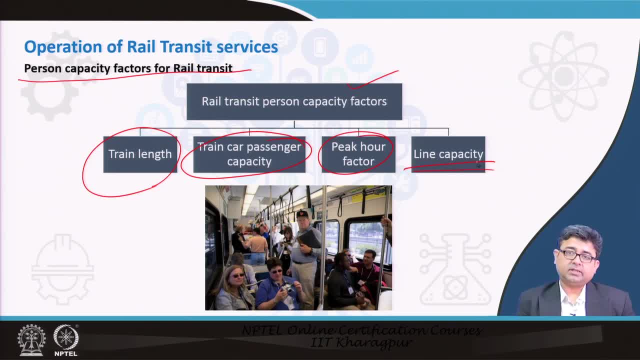 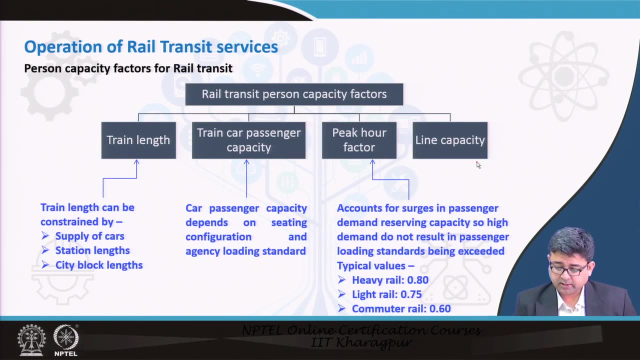 factor and, of course, the line capacity, whether you have a double line, a single line and even with a single line, how much capacity can you, how much headway can you have between 2 consecutive trains? Train length, you understand. supply of cars: 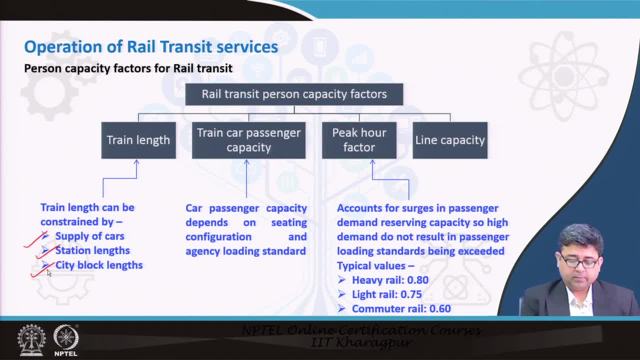 station lengths, city block lengths, number of cars will depend. supply of cars will depend upon how big your city blocks are. if your city blocks are too close to each other, then passengers may get on and off very frequently and you may not need too many cars in your